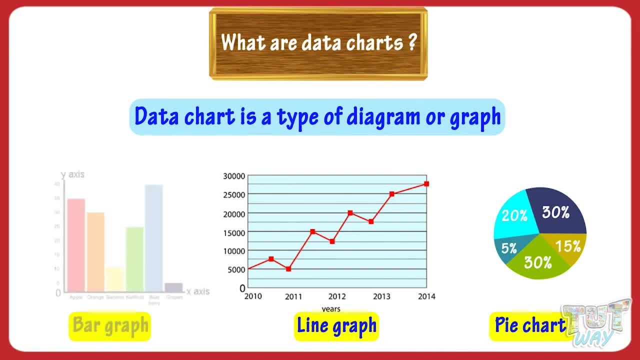 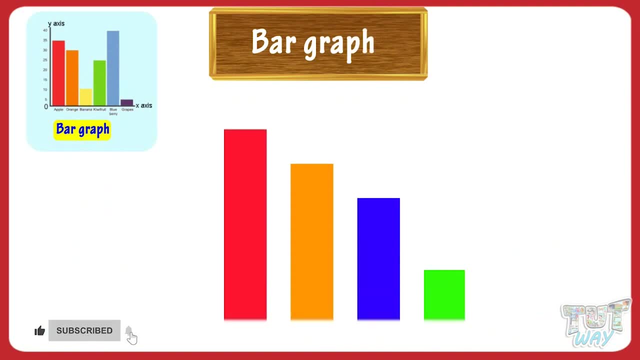 Today we will learn what are bar graphs. A bar chart is a chart with rectangular bars where the length of bars represent the value of something and there is a scale along the length of bars which is used to measure hours measure the length of bars. The bars can be plotted horizontally or vertically. 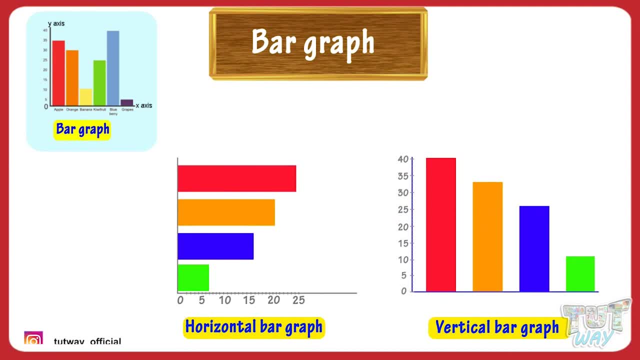 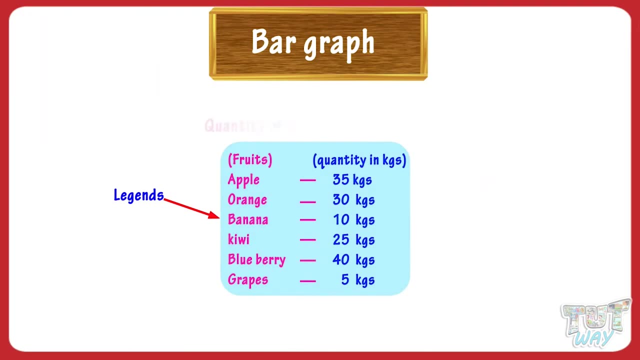 Bar graphs are used to compare the values of given items at any given point of time. Let's learn more about bar graphs using some examples. Here we have some data. A farmer sold different quantities of fruits in a particular month and he recorded the sales, like. 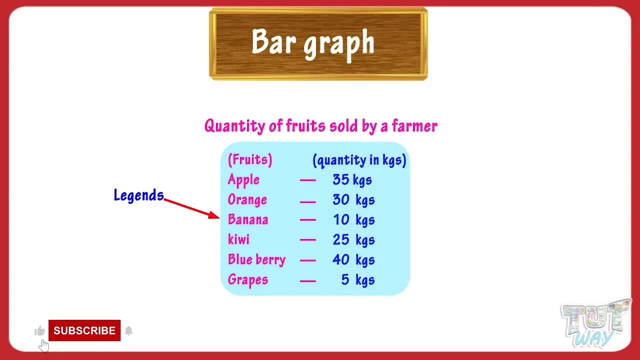 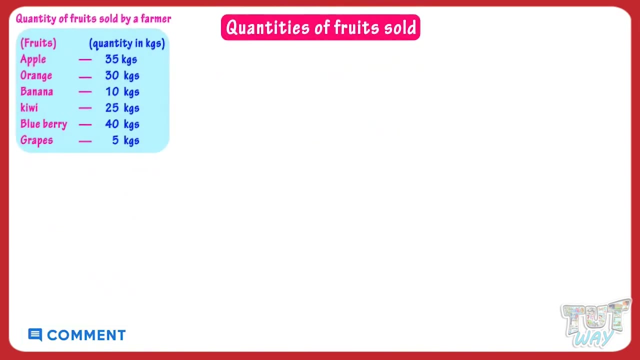 this. Now we will store this data in the form of a bar graph. First of all, determine what will be the title of our bar graph, Like it can be quantities of fruits sold. A bar graph has two attributes: Axis: x-axis and y-axis. We have two types of data. One is the numeric data showing quantities. 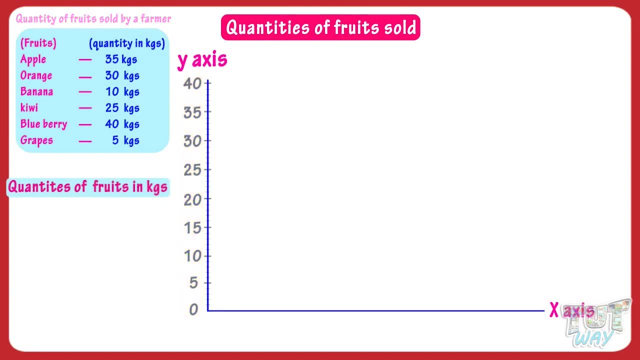 of fruits in kgs and the other is textual data: the name of fruits. The axis which shows numeric data is called scale, As on the y-axis we are showing the numeric data And our numeric data is in the range of 1 to 40. So make a scale showing numbers 1 to 40.. 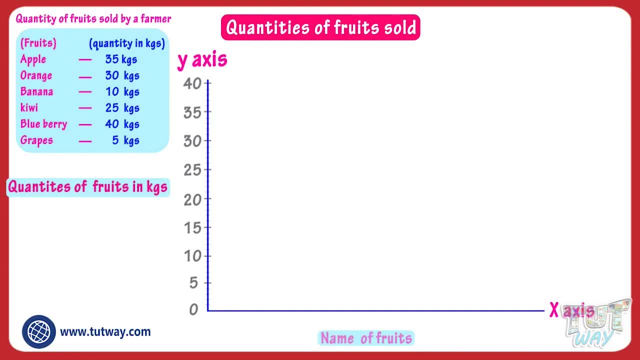 Now, on x-axis, we will show the names of fruits and we'll also relate them to their quantities. Like it's given that 35 kgs of apples were sold, So make a rectangular bar up to the mark of fruits And make one of these numbers a percent of 30. and sign it with apples. 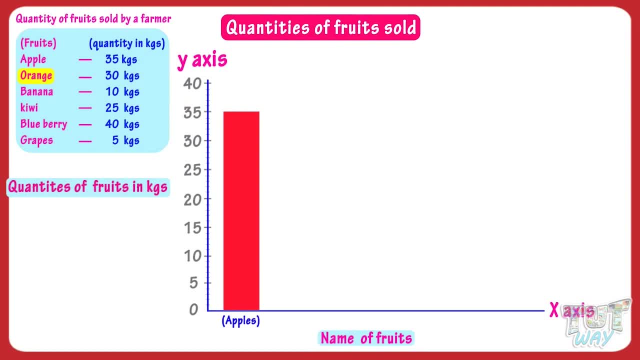 Now, next fruit is Orange. Quantity of oranges sold is 30 kgs, So make a rectangular bar up to the mark of 30 and label it with oranges. Now, next fruit is Banana. Quantity of bananas sold is 10 kgs, So make a rectangular bar up to the mark of 30.. 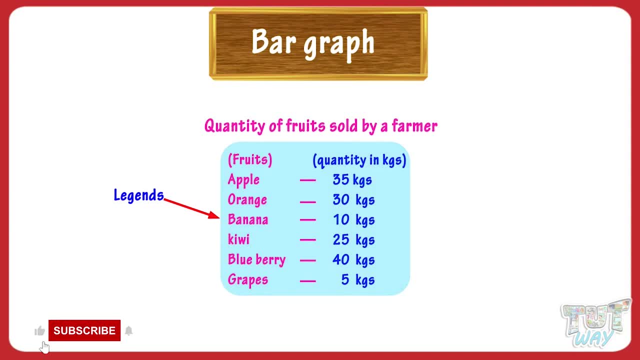 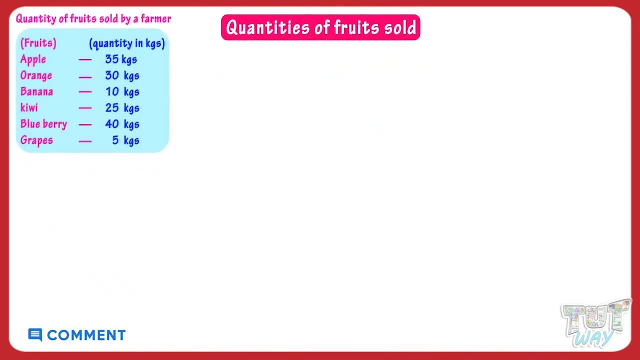 this. Now we will store this data in the form of a bar graph. First of all, determine what will be the title of our bar graph, Like it can be quantities of fruits sold. A bar graph has two attributes: Axis: x-axis and y-axis. We have two types of data. One is the numeric data showing quantities. 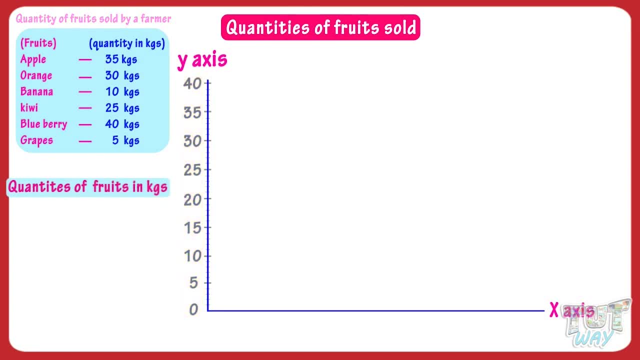 of fruits in kgs and the other is textual data: the name of fruits. The axis which shows numeric data is called scale, As on the y-axis we are showing the numeric data And our numeric data is in the range of 1 to 40. So make a scale showing numbers 1 to 40.. 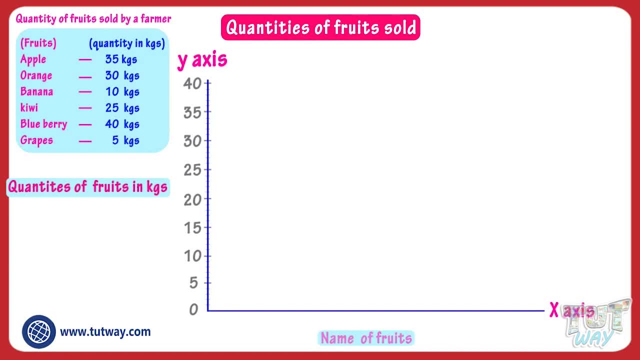 Now, on x-axis, we will show the names of fruits and will also relate them to their quantities, Like it's given that 35 kgs of apples were sold. So make a rectangular bar up to the mark of fruits And label it with apples. Our next fruit is orange. Quantity of oranges sold is 30 kgs. So 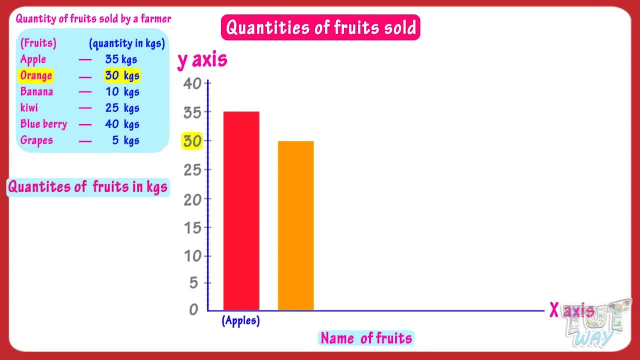 make a rectangular bar up to the mark of 30 and label it with oranges. Now next fruit is banana. Quantity of bananas sold is 10 kg's. So make a rectangular bar up to the mark of 30. min of 10- and label it with banana. now the next fruit is kiwi. the quantity sold is 25 kgs. 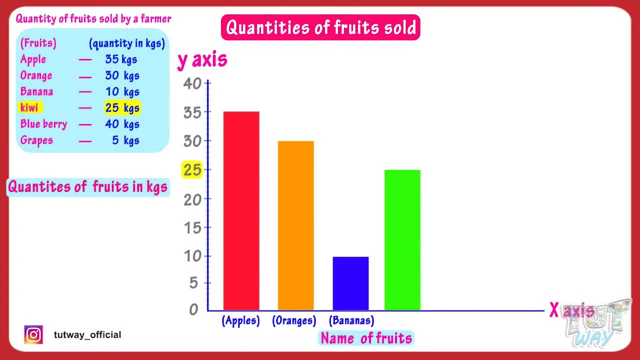 so make a rectangular bar up to the mark of 25 and label it with kiwi now. next fruit is blueberry. its quantity sold is 40 kgs. so make a rectangular bar up to the mark of 40 and label it with blueberry now. next fruit is grapes, and the quantity sold is 5 kgs. 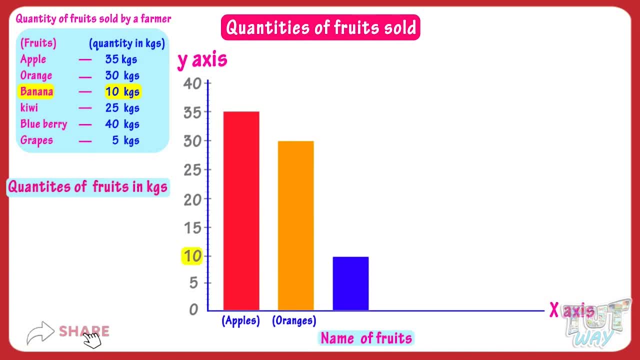 Or a fur dependant, is 30 in the enduring length, similar to the picture that I described earlier. And here we give classes to eggs. This comes from the same example as we use rainy season scene of 10 and label it with banana. now the next fruit is kiwi. the quantity sold is 25 kgs. 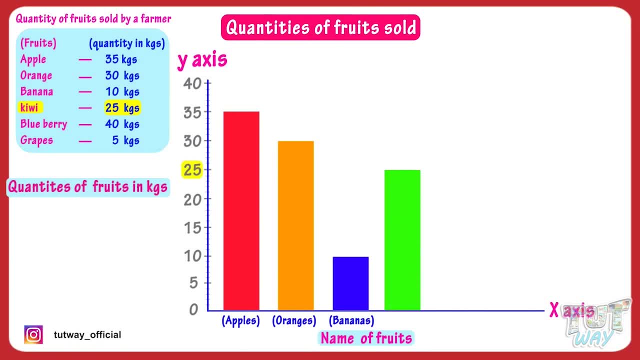 so make a rectangular bar up to the mark of 25 and label it with kiwi now. next fruit is blueberry. its quantity sold is 40 kgs. so make a rectangular bar up to the mark of 40 and label it with blueberry now. next fruit is grapes, and the quantity sold is 5 kgs. so make 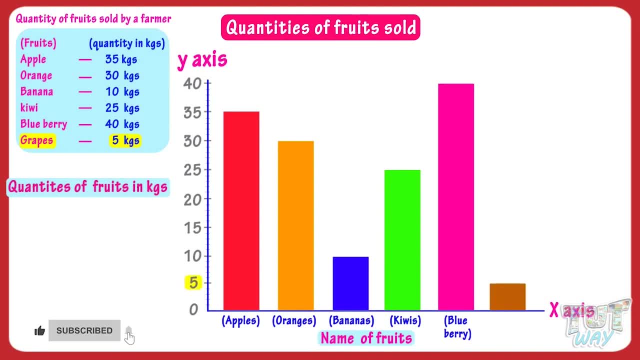 a rectangular bar up to the mark of 5 and label it with grapes, and our bar graph is ready. this is a graph we just made. now let's read it here. the bars are drawn vertically on horizontal axes. this axis is known as horizontal axes or x-axis. the length rectangular bars are represent. 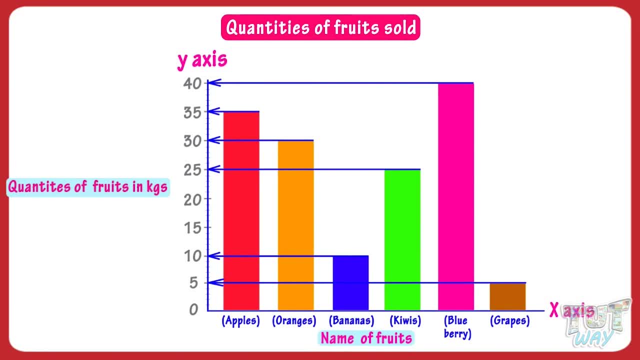 the quantities of corresponding fruits sold in kgs. length of the bars is measured with the vertical scale along the vertical axes or y-axis, as the numerical data is give on the vertical axes. this axis is the vertical axes, which shows 35 kgs of apples sold. quantity of: 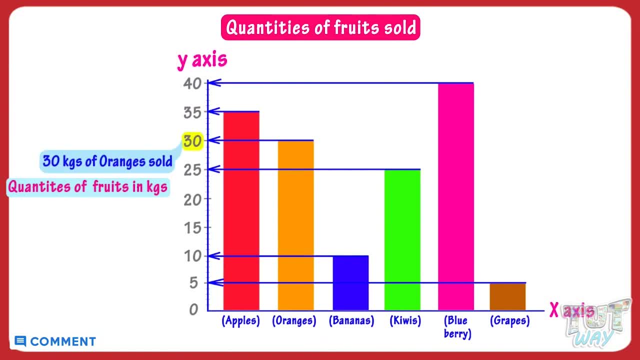 oranges sold is 30 kgs. quantity of bananas sold is 10 kgs. Blueberries are sold the most, Bananas are sold the least. so kids data in the form of charts is much easier to read and Represent. it is easier to compare data values. Now let's see another example. 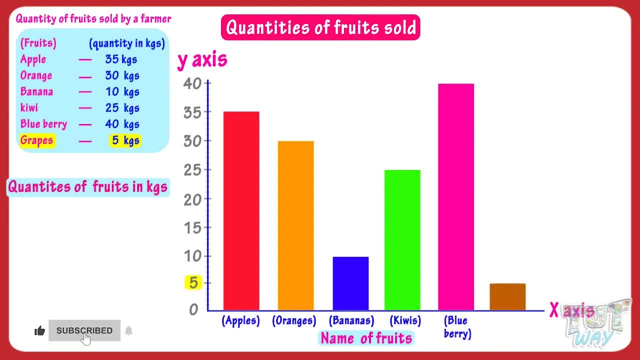 so make a rectangular bar up to the mark of 5 and label it with grapes, and our bar graph is ready. this is a graph we just made. now let's read it here. the bars are drawn vertically on horizontal axes. this axis is known as horizontal axes or x-axis. the length rectangular bars are represent. 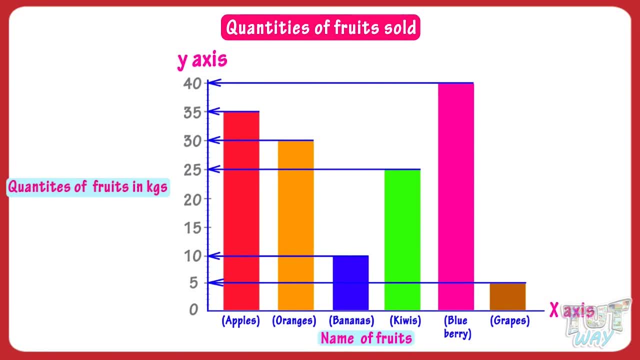 the quantities of corresponding fruits sold in kgs. length of the bars is measured with the vertical scale along the vertical axes or y-axis, as the numerical data is give on the vertical axes. this axis is the vertical axis which shows 35 kgs of apples sold. 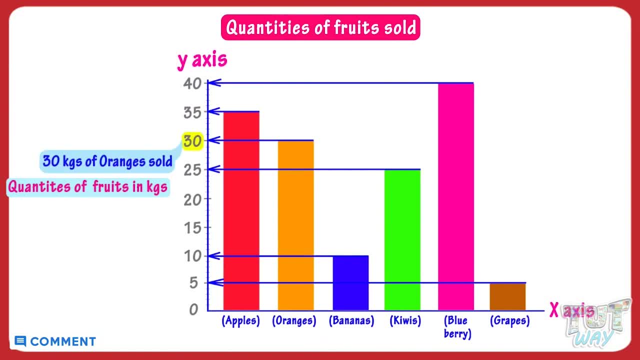 quantity of oranges sold is 30 kgs. quantity of bananas sold is 10 kgs. the horizontal axis is remaining the vertical axis is. the vertical axis part of the horizontal axis, where 2 and 1 are showing the width of the bars and singleton bar, and the horizontal axis is 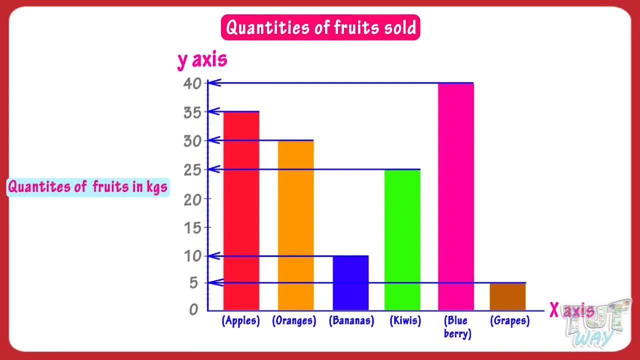 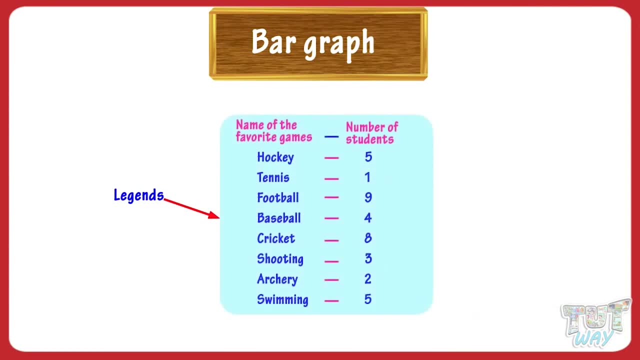 the vertical axis and a long vertical axis is showing the width of the bars, walls, and left area is the vertical axis. many people think if you're just thinking those different connectors. but that's actually not true. they must be from the extreme north. so let's, poor polygons, have things quiet and straight and nice and simple and all right, let us move to the middle. we have next results. 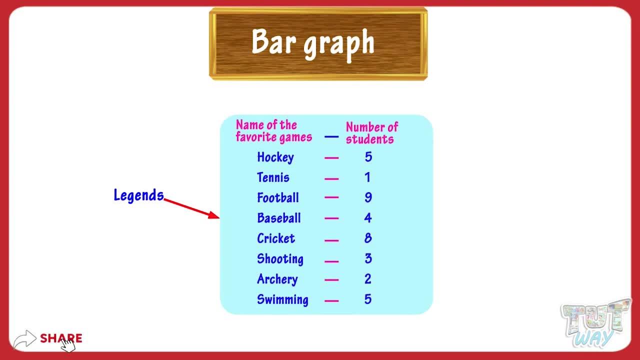 so blue. so let's make sure that each of banana plus l in total and banana plus l of l and banana plus l is disputed. Note it down like this: 5 students like hockey the most. That is, the favorite game of 5 students is hockey. 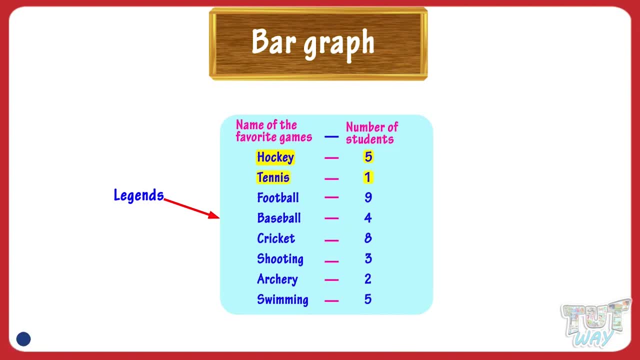 Favorite game of 1 student is tennis, Favorite game of 9 students: football, and so on. Now let's see how it can be represented in the form of a bar graph. We have two types of information. One is the numeric values, given the number of students. 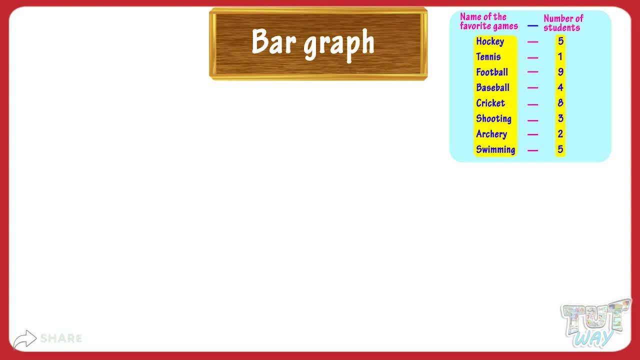 One is textual values given the names of their favorite game. First of all, we can give a title to our chart. It can be choice of games in a class. We can give titles to each axes of graph. Let's see how it can be represented. 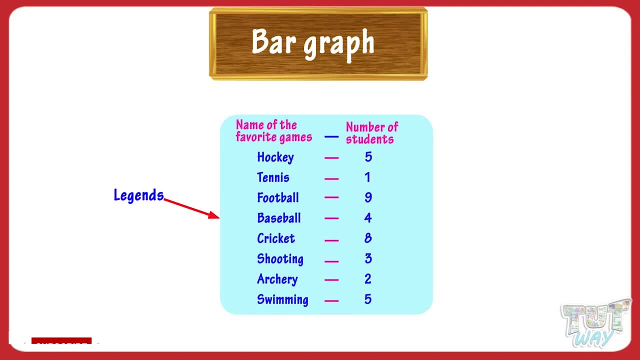 We are given with another data from a class of students. Favorite game of each student was asked and noted down like this: by students like hockey the most, That is, a favorite game of five students is hockey. Favorite game of one student is tennis. Favorite game of nine students: football, and so on. 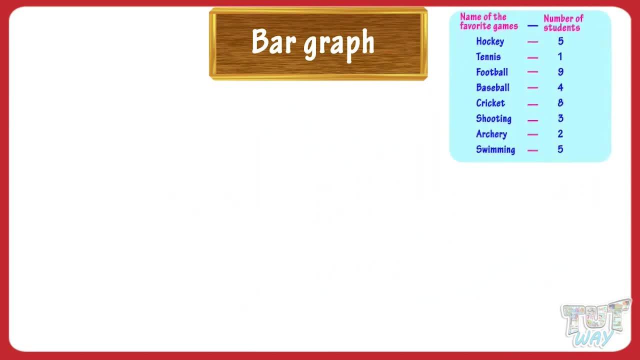 Now let's see how it can be Represented in the form of a bar graph. We have two types of information. One is the numeric values, given the number of students. One is textual values, given the names of their favorite game. first of all, we can give a title to our chart. it can be: 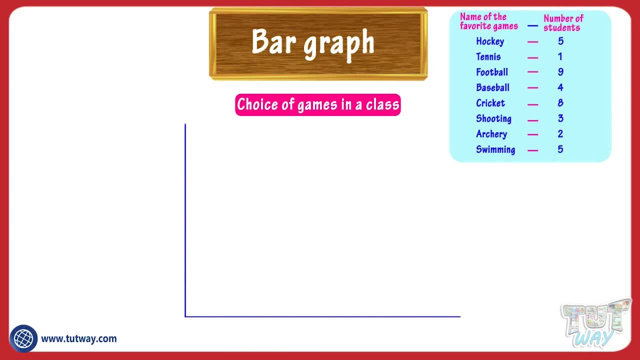 choice of games in a class. We can give titles to each axis of graph. Let X axis be number of students. Let Y axis be name of the favorite game. X axis represents the number of students, so it will be the scale. Number of students is in the range of 1 to 9.. So let the scale be numbered 1 to 10.. 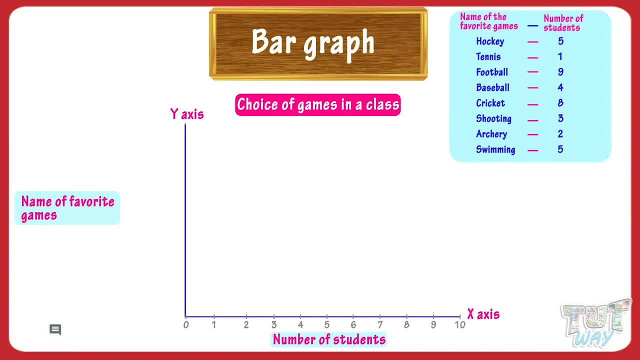 Now on Y axis will show the names of games and we will also relate them to the number of students whose favorite game it is Like. it's given that five students like swimming the most, So make a rectangular bar on Y axis up to the mark of five and label it with swimming. 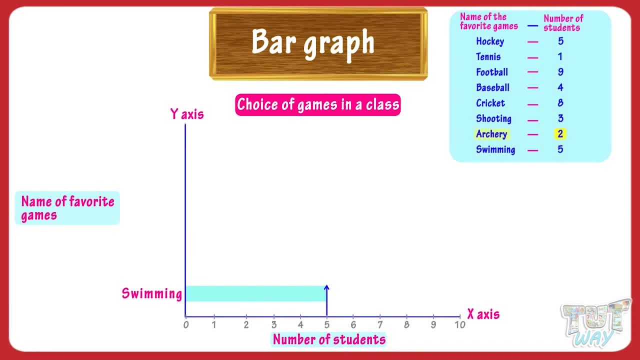 Now it's given that two students like archery the most, So make a rectangular bar on Y axis up to the mark of two and label it with archery. Now it's given that five students like swimming the most, So make a rectangular bar on Y axis up to the mark of five and label it with archery. Now it's given that five students like swimming the most, So make a rectangular bar on Y axis up to the mark of two and label it with archery. Now it's given that five students like swimming the most, So make a rectangular bar on Y axis up to the mark of two and label it with archery. 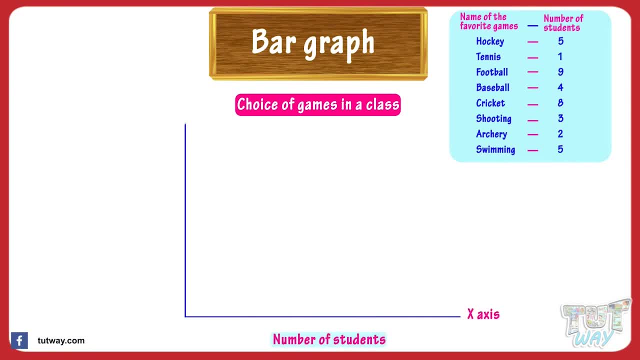 Let x-axis be number of students. Let y-axis be name of the favorite game. X-axis represents the number of students, so it will be the scale. Number of students is in the range of 1 to 9.. So let the scale be numbered 1 to 10.. 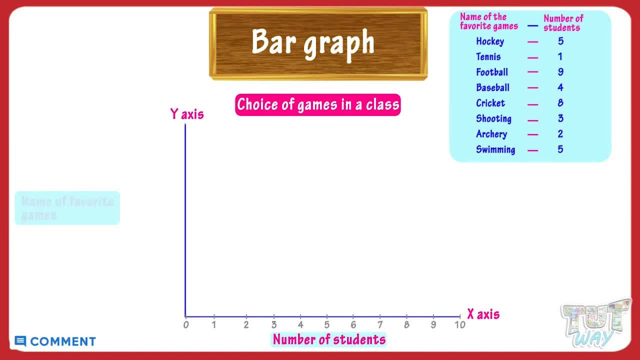 Now on y-axis, will show the names of the favorite games. Now on, the x-axis will show the names of the favorite games- names of games- and we will also relate them to the number of students whose favorite game it is like. it's given that five students like swimming the most, so make a rectangular bar. 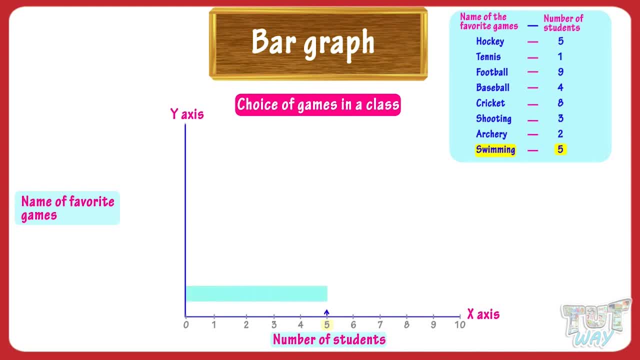 on y-axis up to the mark of five and label it with swimming. now it's given that two students like archery the most, so make a rectangular bar on y-axis up to the mark of two and label it with archery. now it's given that three students like 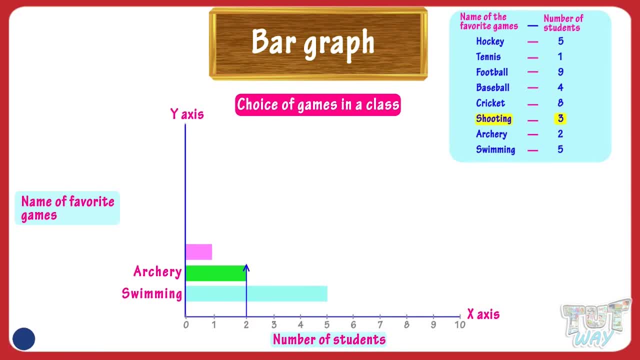 shooting the most, so make a rectangular bar on y-axis up to the mark of three and label it with archery shooting. now it's given that eight students like cricket the most, so make a rectangular bar on y-axis up to the mark of eight and label it with cricket. similarly, we can draw bars for all. 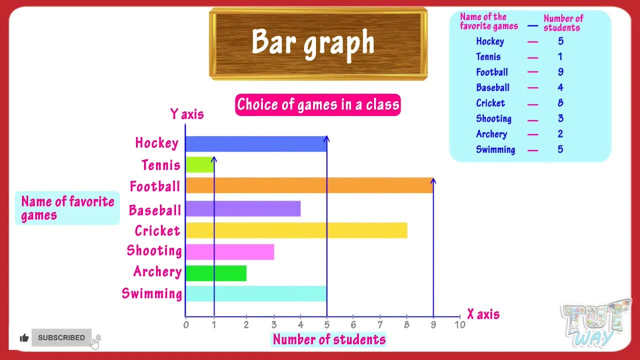 and our graph will be ready. this is a graph where the rectangular bar are drawn horizontally on the bottom right of the bar and the bottom left of the bar, and then down on the left side of the bar, and then down on the right side of the bar and then up on the left side of the bar. 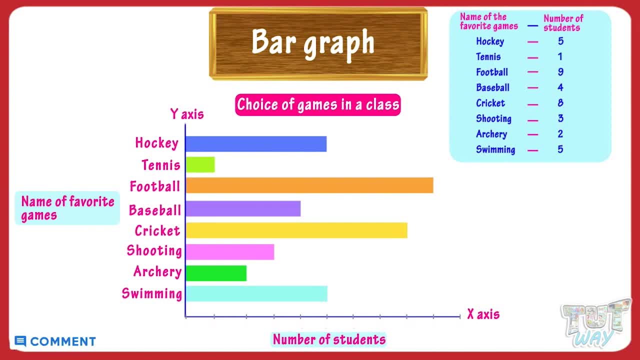 the y-axis and the scale is drawn on the x-axis. Let's read the graph. Graph shows that the favorite game of students is football, as the bar corresponding to football is the longest and the length of bar is nine, That is, nine students like football. Least favorite game. 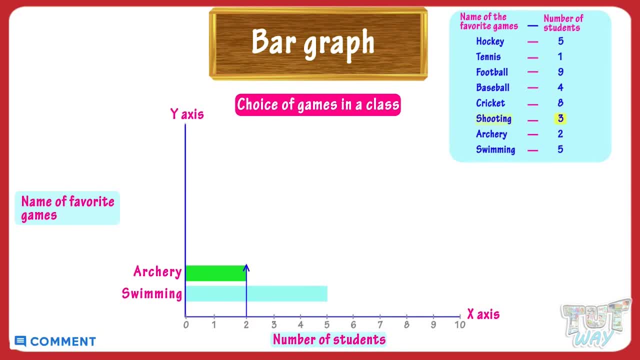 Now it's given that five students like swimming the most, So make a rectangular bar on Y axis up to the mark of two and label it with archery. Now it's given that 3 students like shooting the most, so make a rectangular bar on y-axis up to the mark of 3, and label it with shooting. 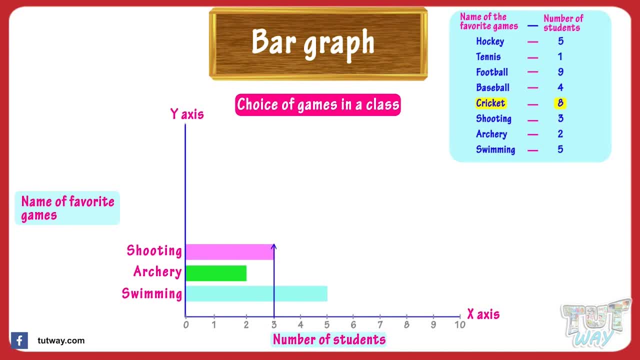 Now it's given that 8 students like cricket the most, so make a rectangular bar on y-axis up to the mark of 8, and label it with cricket. Similarly, we can draw bars for all and our graph will be ready. 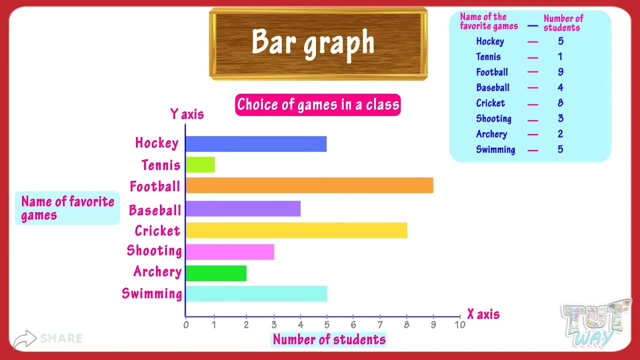 This is a graph where the rectangular bar are drawn horizontally on the y-axis and the scale is drawn on the x-axis. Let's read the graph. The graph shows that the favorite game of students is football, As the bar corresponding to football is the longest and the length of bar is 9.. 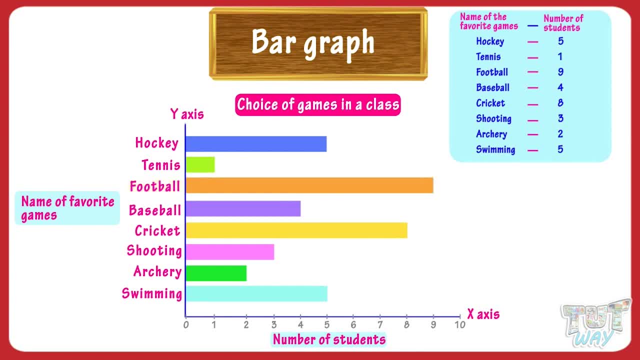 That is, 9 students like football. Least favorite game of students in the class is tennis, and only 1 student likes tennis the most. Second most favorite game in the class is cricket, as 8 students like cricket the most. So kids. 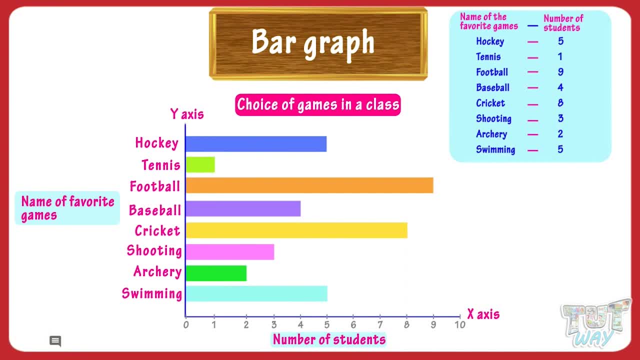 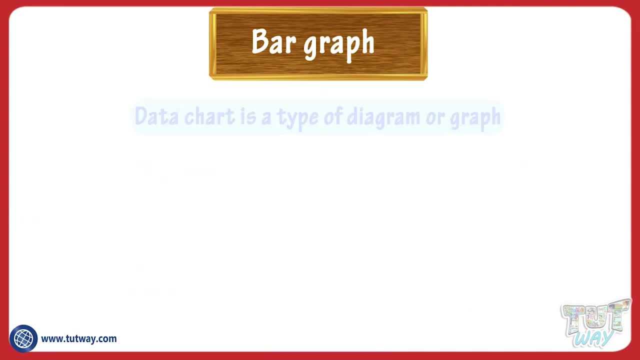 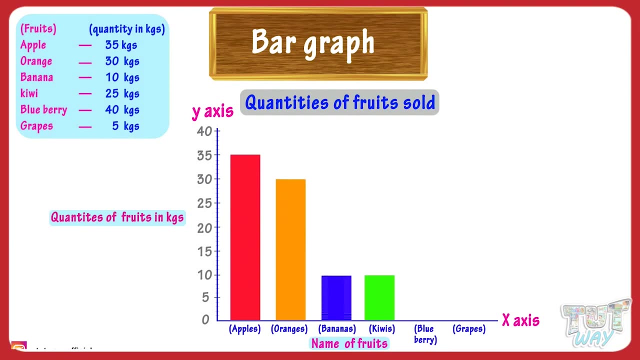 Data represented in the form of a bar graph is easy to read. So, kids, today we learned what are data charts and learned how to make a bar graph out of the given data. Also, how to read a bar graph. Now go ahead and take a quiz to learn more. 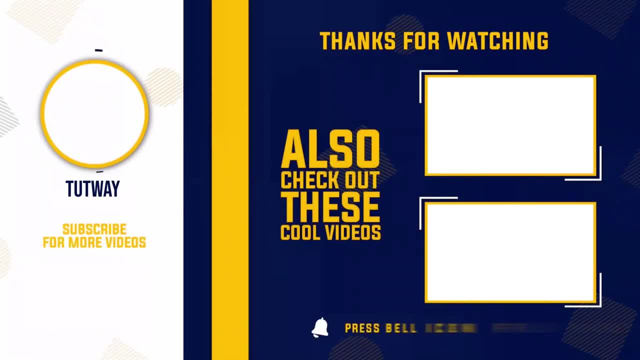 Bye, bye. Thank you so much for watching. Don't forget to like, comment and share this video, and if you want to see more fun videos, you can hit that subscribe button. You can also follow us on Facebook and Instagram for more content. Bye, bye.